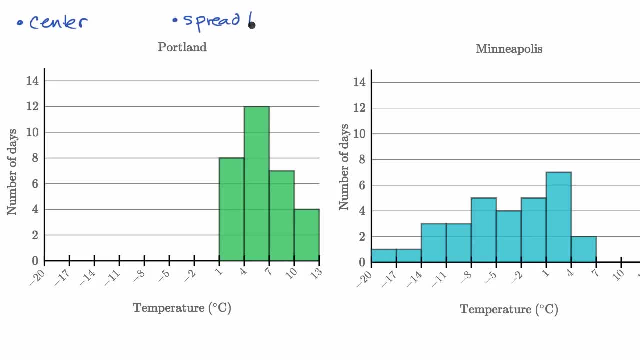 and also the spread. Sometimes people will talk about the variability of the distributions, And so these are the things that we're going to compare, And in making the comparison, we're actually just going to try to eyeball it. We're not gonna try to pick a measure of central tendency. 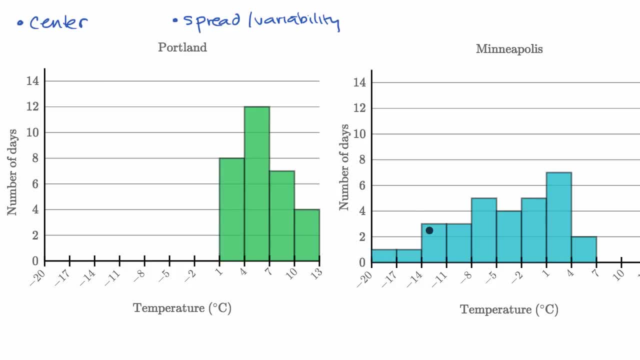 say the mean or the median, and then calculate precisely what those numbers are for these. We might wanna do those if they're close, but if we can, if we can just eyeball it, that would be even better. Similar for the spread and variability. 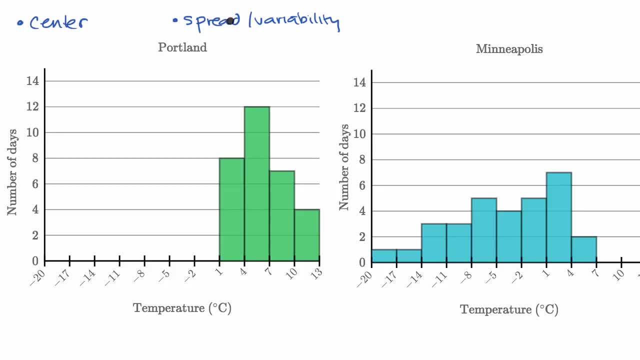 In either of these cases there are multiple measures in our statistical toolkit Center. mean median is valuable for the center For spread variability. the range, the interquartile range, the mean absolute deviation, the standard deviation, these are all measures. 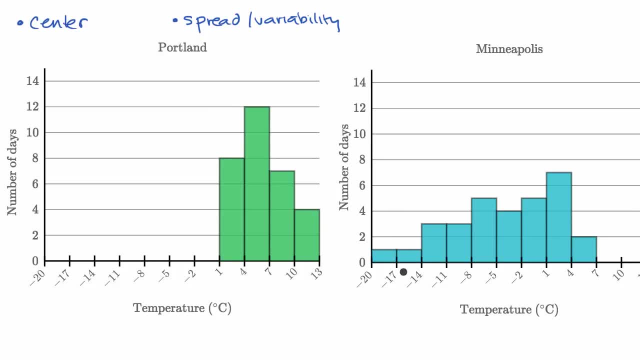 But sometimes you can just kind of gauge it by looking. So, in this first comparison, which distribution has a higher center, Or are they comparable? Well, if you look at the distribution for Portland, the center of this distribution, let's say, if we were to just think about the mean, 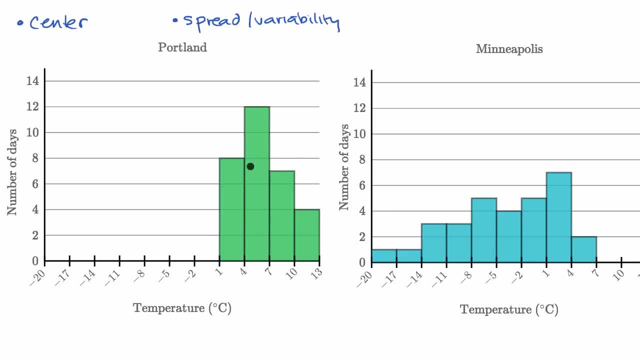 although I think the mean and the median would be reasonably close right over here. It seems like it would be around. it would be around seven or maybe a little bit lower than seven, So it would be kind of in. it'd be kind of in that range. 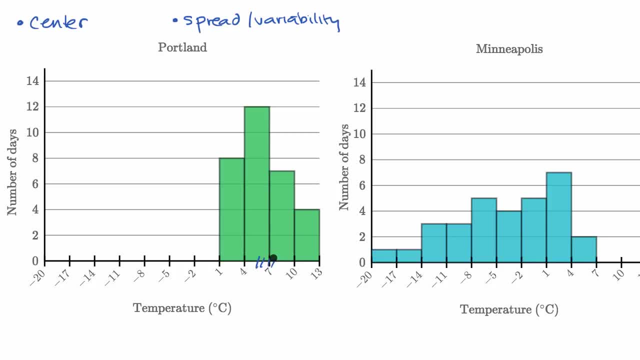 maybe between five and seven would be. our central tendency would be either our mean or our median, While for Minneapolis it looks like our center is much closer to maybe negative two or negative three degrees Celsius. So here, even though we don't know precisely, 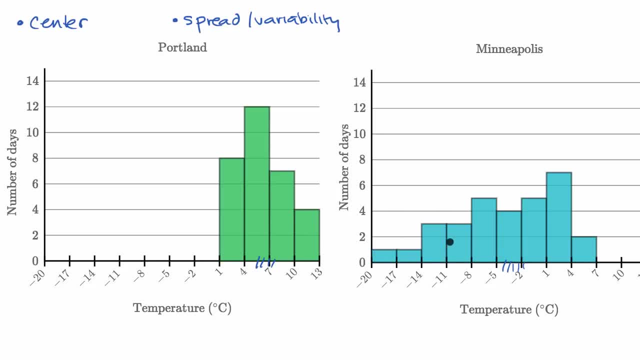 what the mean or the median is of each of these distributions. you can say that Portland- Portland distribution has a higher center. However, you want to measure it, either mean or median. Now, what about the spread, or variability? Well, if you just superficially thought about range, 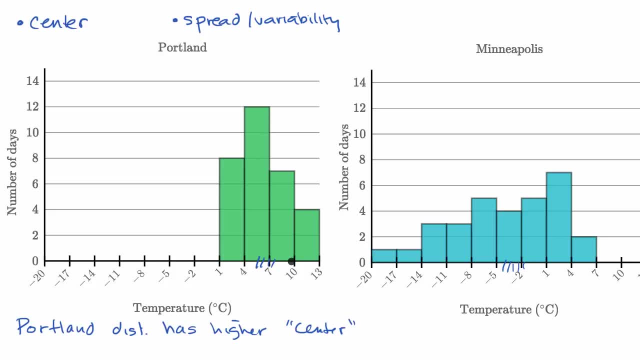 you see here that there's nothing below one degree Celsius and nothing above 13,. so you have about a 13 degree range at most right over here. In fact, what might be contributing to this first column? it might be a bunch of things at three degrees. 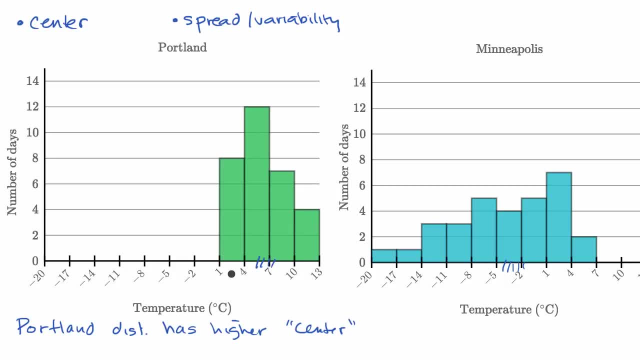 or even 3.9 degrees and similarly. it might be a bunch of things at three degrees, or even 3.9 degrees, and similarly it might be a bunch of things at three degrees and similarly. what's contributing to this last column? 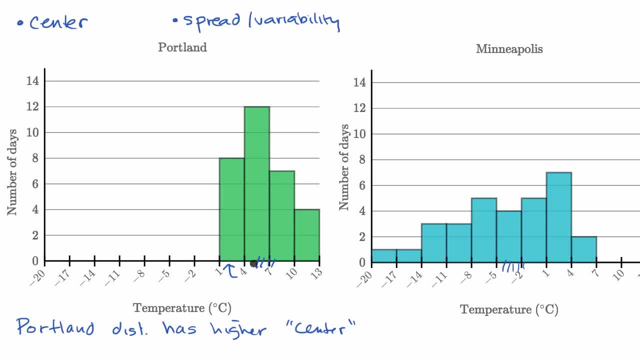 might be a bunch of things at 10.1 degrees, but at most you have a 12 degree range right over here, while over here it looks like you have. well, it looks like it's approaching a 27 degree range. 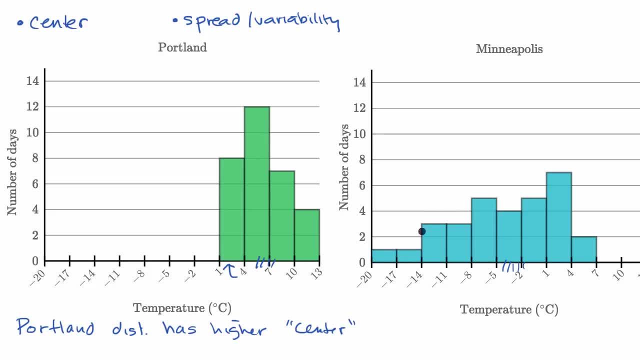 So, based on that, and even if you just eyeball it, this is just we're using the same scales for our horizontal axes here, the temperature axes, and this is just a much wider distribution than what you see over here, And so you would say that the Minneapolis distribution 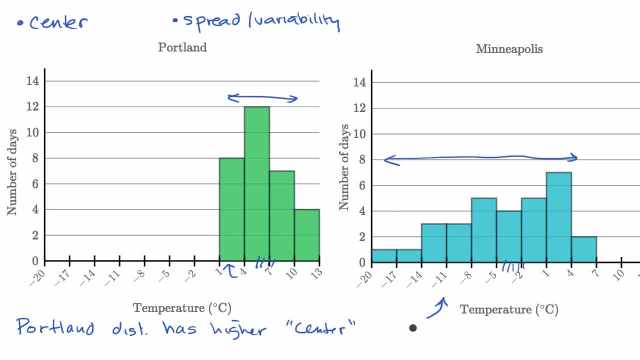 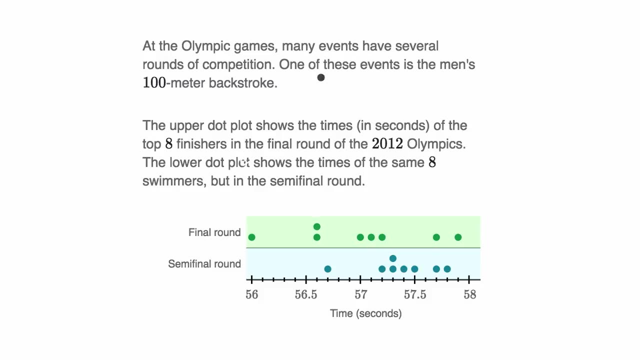 has more spread or higher spread or more variability. So higher spread, right over here. Let's do another example and we'll use a different representation for the data here. So we're told, at the Olympic Games many events have several rounds of competition. 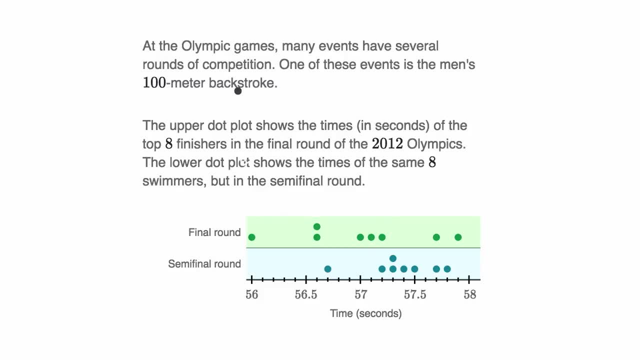 One of these events is the men's 100 meter backstroke. The upper dot plot shows the times in seconds of the top eight finishers in the final round of the 2012 Olympics. So that's in green right over here, the final round. 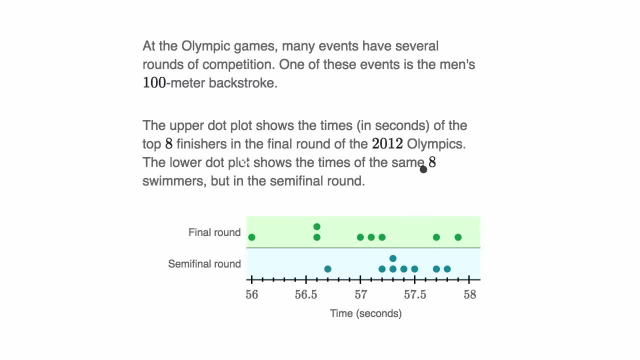 The lower dot plot shows the times of the same eight swimmers, but in the semifinal round. So, given these distributions, which one has a higher center? Well, once again, I mean, and here you can, actually it's a little bit easier to eyeball. 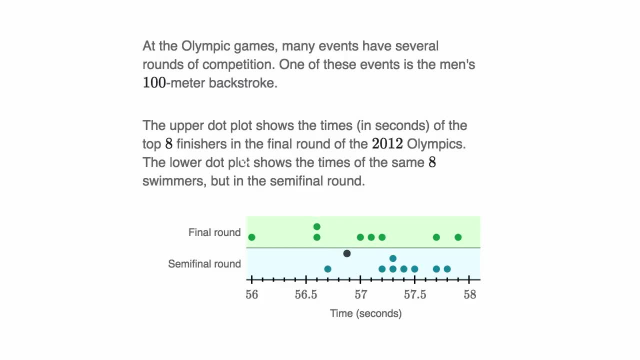 even what the median might be. The mean, I would probably have to do a little bit more mathematics, But let's say the median. let's see one, two, three, four, five, six, seven, eight data points. 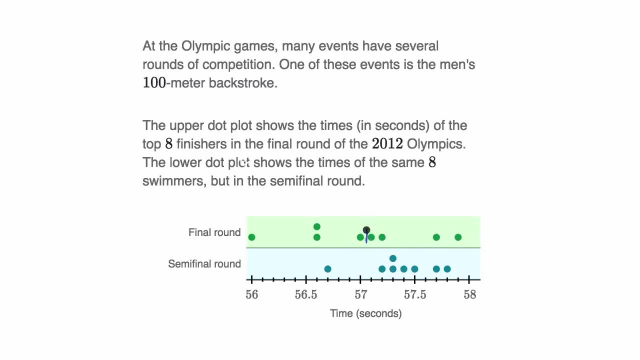 So the median is gonna sit between the lower four and the upper four. So the central tendency right over here is for the final round looks like it's around 57.1 seconds, especially if we think about the median, While the central tendency for the semifinal round 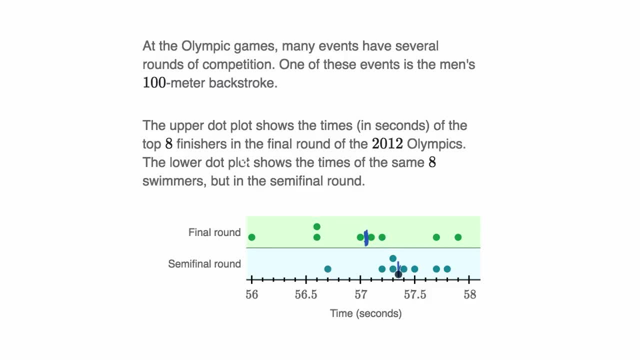 let's see one, two, three, four, five, six, seven, eight. looks like it is right about there. So this is about 57, more than 57.8 seconds. Three seconds, So the semifinal round. 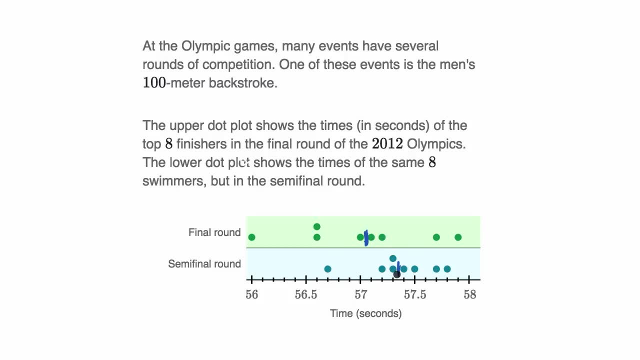 seems to have a higher central tendency, which is a little bit counterintuitive. You would expect the finalist to be running faster on average than the semifinalist, but that's not what this data is showing. So the semifinal round has higher center. 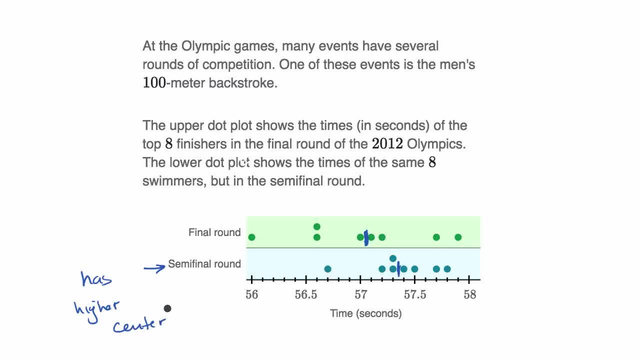 higher, higher center. And I just eyeballed the median And I suspect that the mean would also be higher in this second distribution. And now, what about variability? Well, once again, if you just looked at range, and these are both at the same scale. 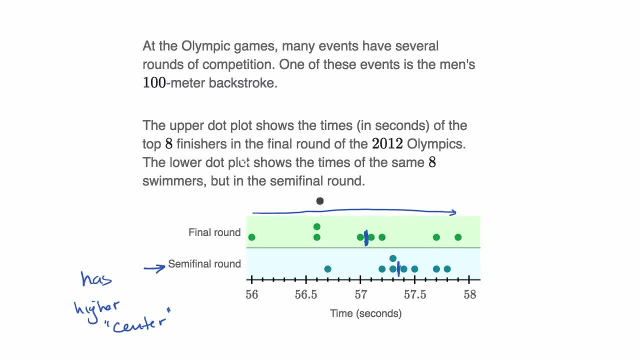 if you just visually look the variability here, the range for the final round is larger than the range for the semifinal round. So you would say that the final round has higher variability, Variability. it has a higher range, Eyeballing it. 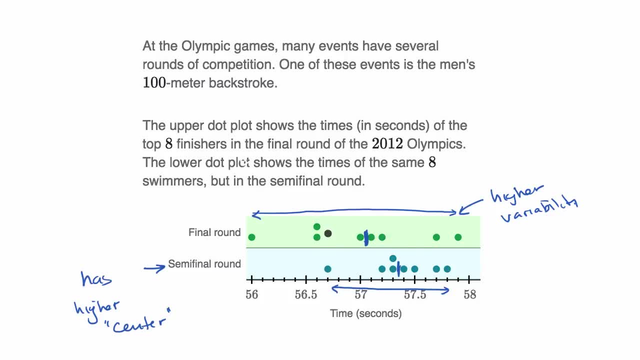 it looks like it has a higher, a higher spread, And there is, of course, times where one distribution could have a higher range, but then it might have a lower standard deviation, For example. you could have data. that's like you know. 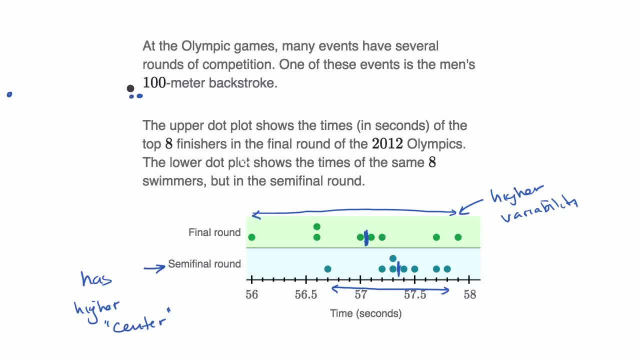 two data points that are really far apart, but then all of the other data just sits right. It's really really closely packed. So, for example, a distribution like this- and I'll draw the horizontal axis here just so you can imagine it as a distribution- 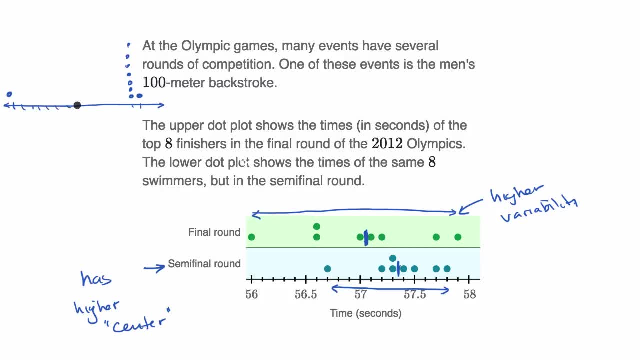 A distribution like this might have a higher range but lower standard deviation than a distribution like this. Let me just- I'm just drawing a very rough example. A distribution like this has a lower range but actually might have a higher standard deviation. might have a higher standard deviation. 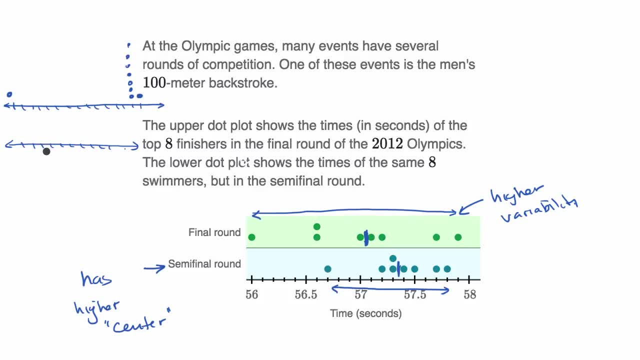 than the one above it. In fact, I can- even I can- make that even better. A distribution like this would have a lower range, but it would also have a higher standard deviation. So you can't just look at, it's not always the case. 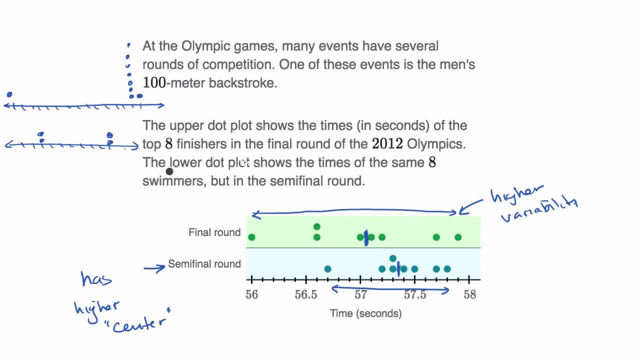 that just by looking at one of these measures, the range or the standard deviation, you'll know for sure. But in cases like this it's safe to say, when you're looking at it by inspection, that look this green. the final round data.